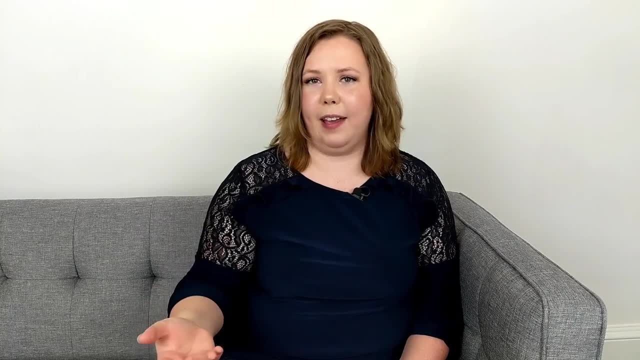 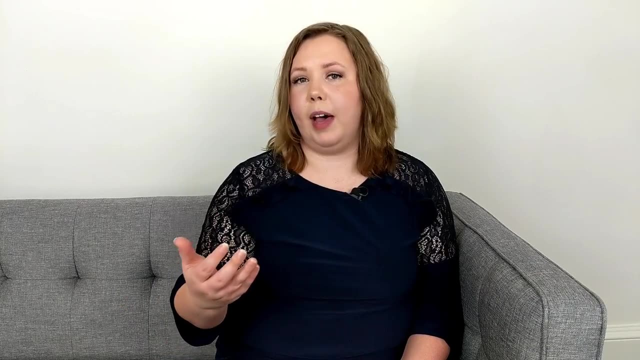 So it takes someone through all the steps of explaining a past situation so that they're able to fully understand it. So when you talk about your analytical skills, you talk about what was the situation where you needed to use them. what were you trying to accomplish, the task that you 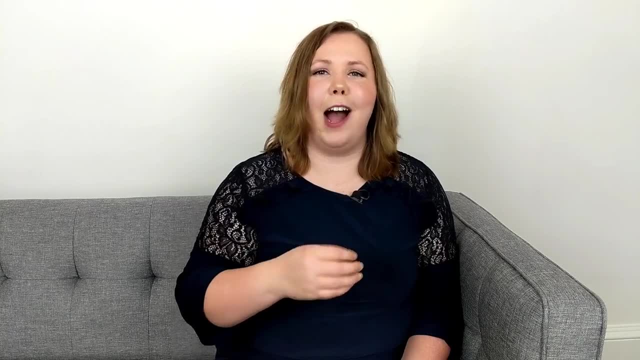 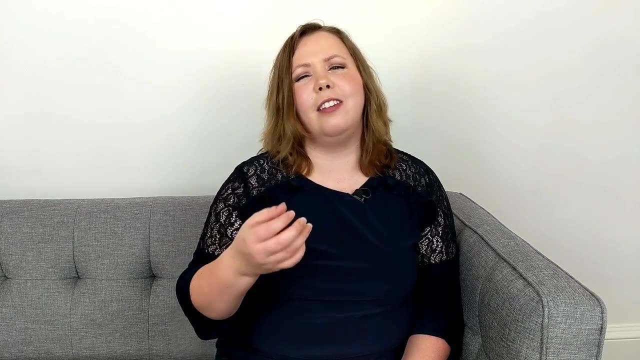 had. So something you're trying to accomplish- solve, figure out whatever word you want to use there, Talk about the steps that you took to solve it, And then you talk about the things that you needed to solve it. So that's where your action is And that's where most of the time in your STAR, 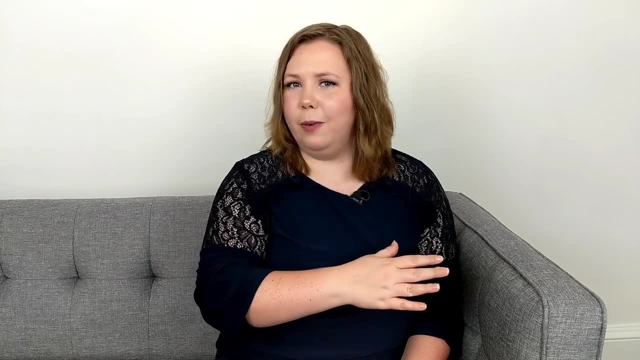 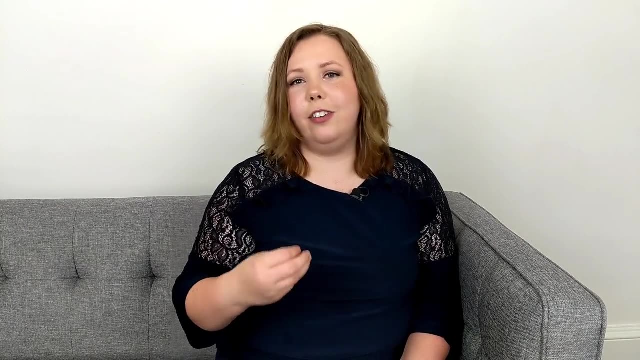 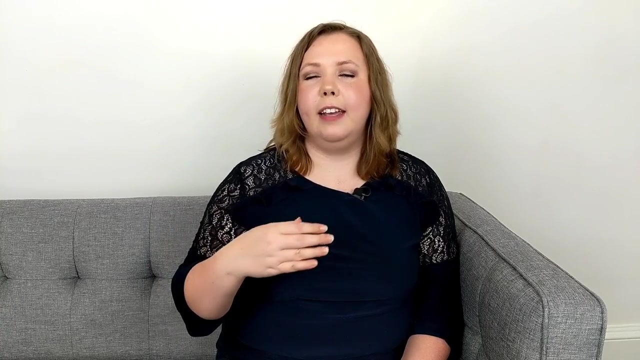 responses should be spent because, regardless of what the background was of what happened and what you were trying to accomplish, what really conveys expertise is what you did. How did you approach solving a problem And whether or not the result was successful? your problem-solving approach is. 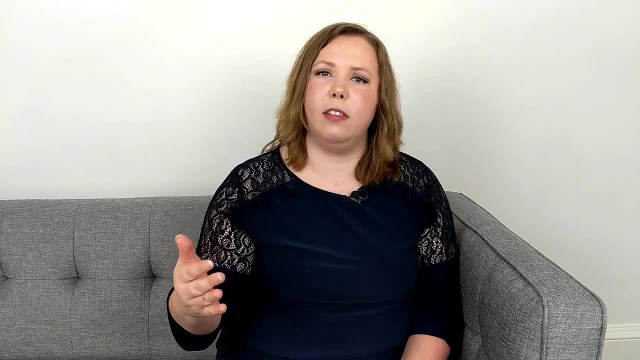 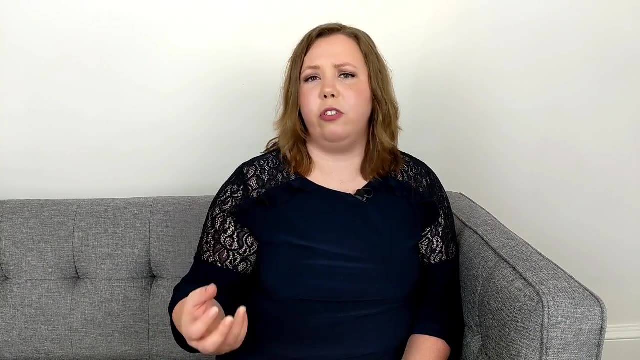 such a crucial aspect of being a good analyst. So explaining that to the interviewer is going to help you understand how you'll be able to solve problems for them in the future or use your analytical skills in the future. So if you want to learn more about how to use the STAR model, I've put a link. 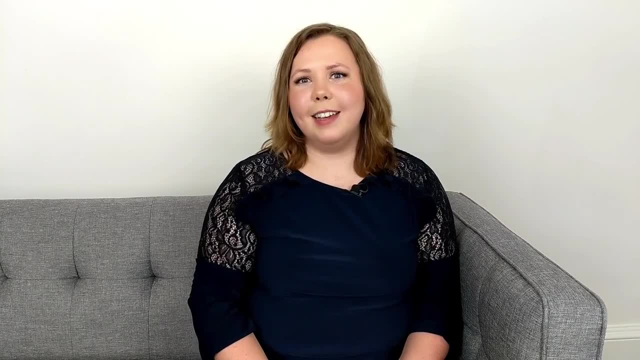 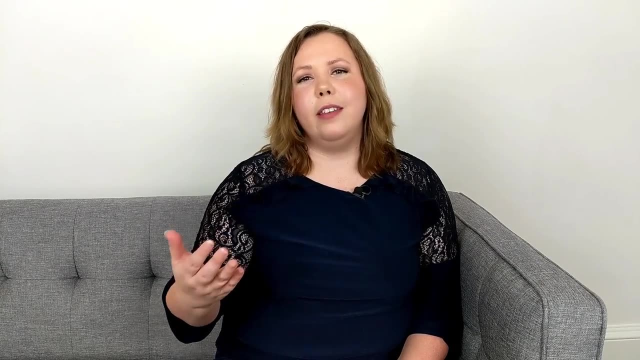 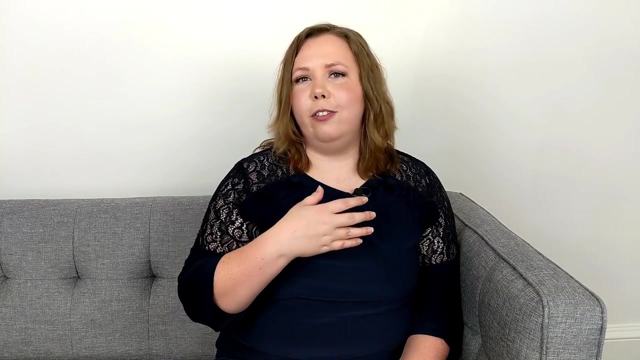 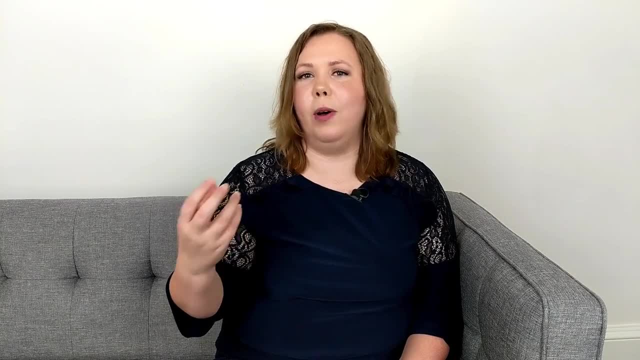 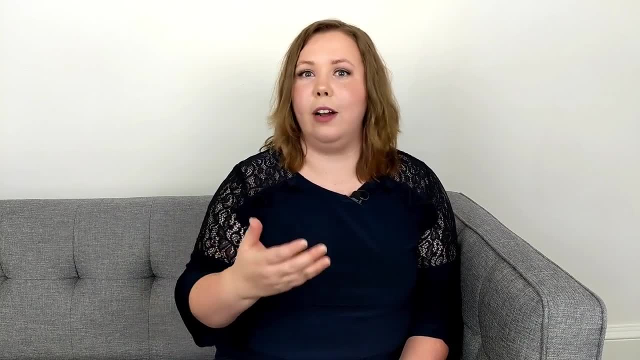 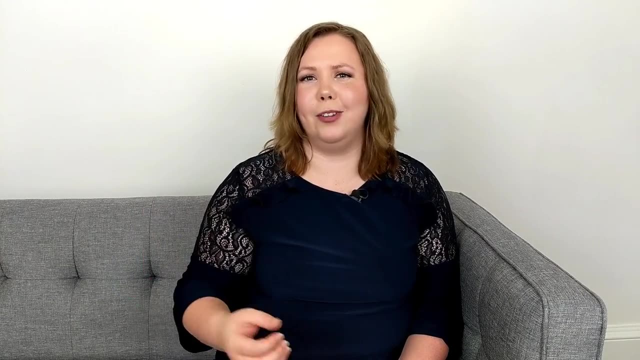 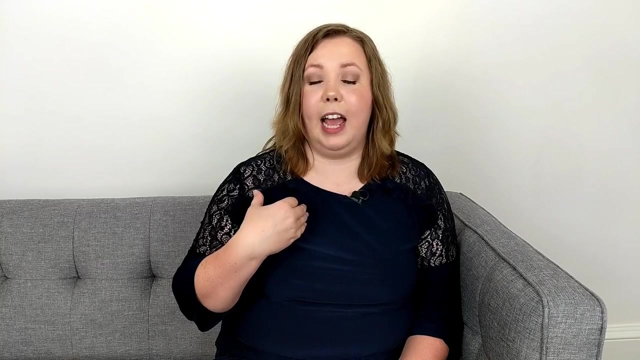 Manhole cover, Round or square or some other shape, And why would we make them round? It could be how many ping pong balls fit on the school bus or something else. So let's look at a specific problem and how I would go about answering it and what I would look for if I was interviewing. 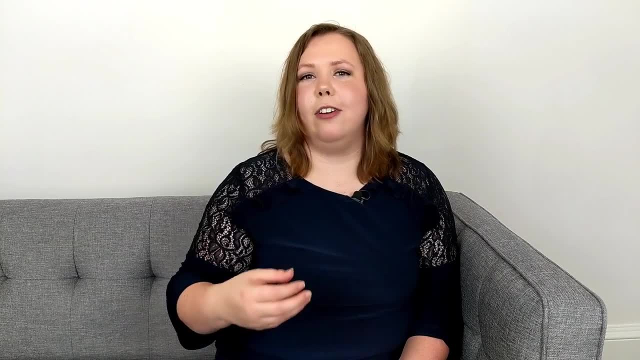 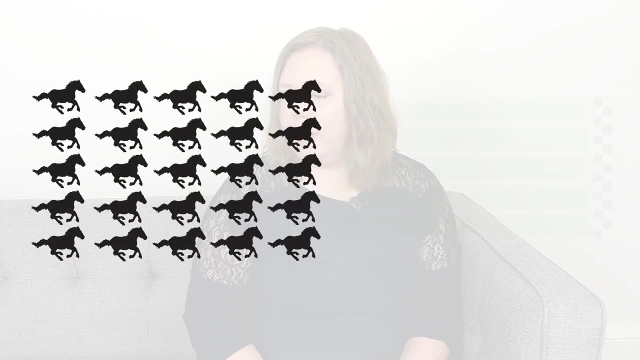 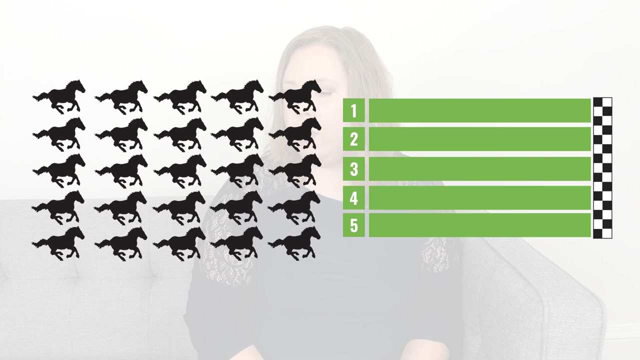 someone to look for a good answer and really be impressed with what they have to say. In this case, we're going to use this example: There are 25 mechanical horses and a single race track. Each horse completes the track in a pre-programmed time and the horses all have. 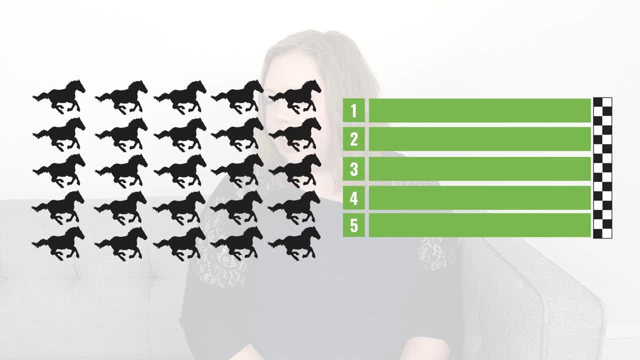 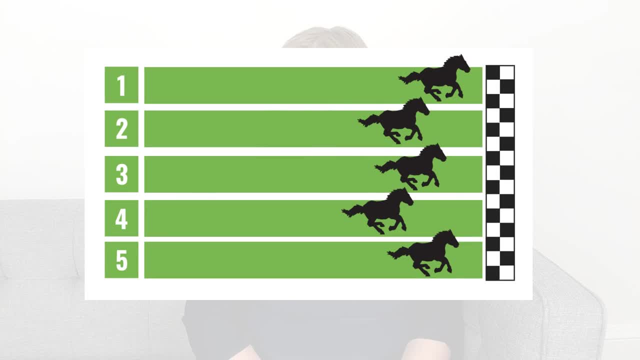 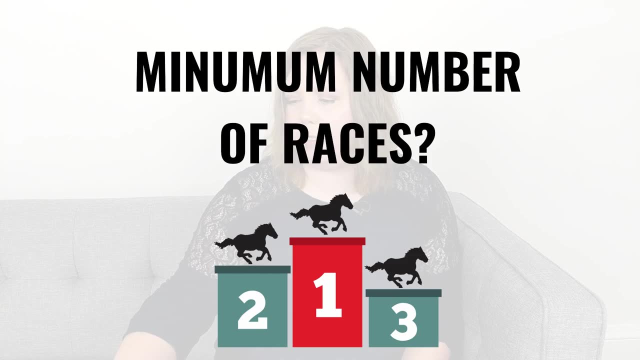 different finishing times, none of which you know. You can race five horses at a time. After a race is over, you get a printout with the order the horse is finished, but not the finishing times of the horses. What is the minimum number of races? you need to identify the fastest three horses. 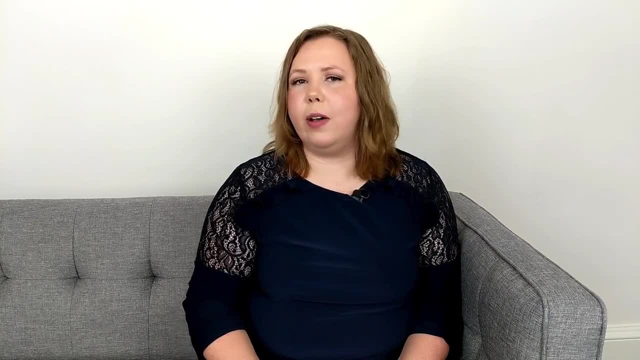 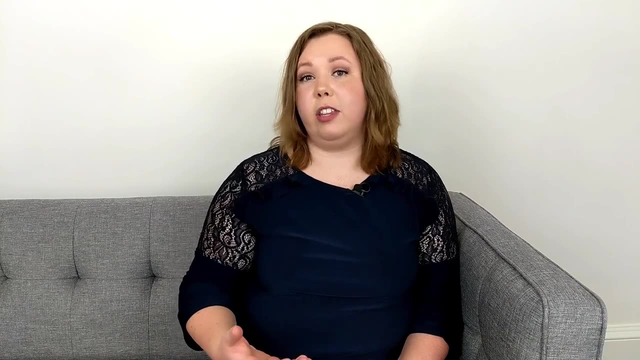 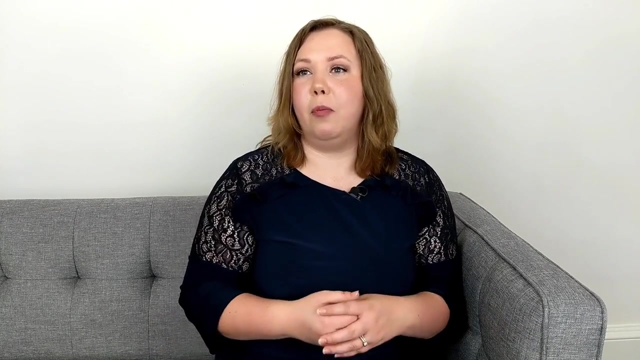 If I were answering this question in an interview, here's how I'd go about answering it. I don't immediately know the answer to it, so I would start talking through the logic that I'm using to figure it out. So I would start out by saying I'm not quite sure how to solve this. 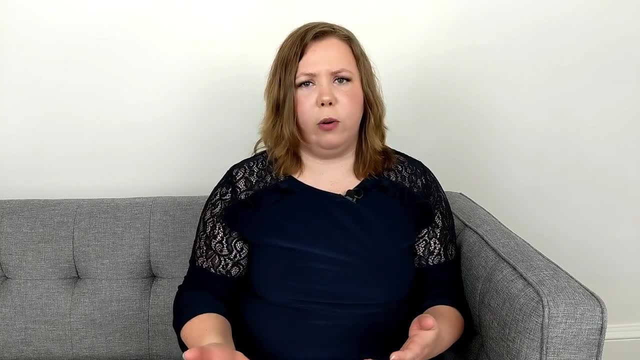 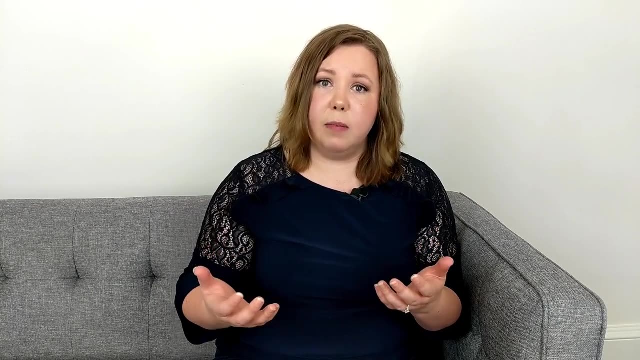 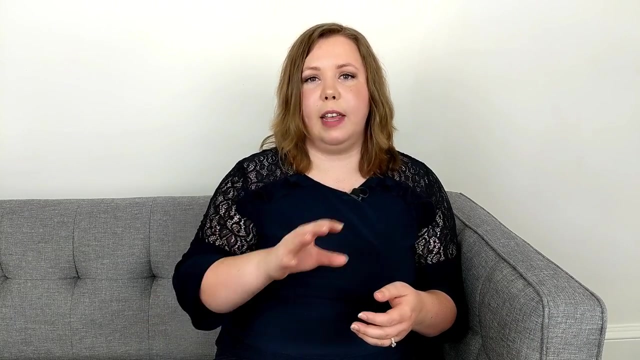 but let me walk you through my logic. I know there's 25 horses and I can race five at the most per race. So I would say, at the minimum I know I need five races to start out so I can find the five fastest horses. I would race each group and say I would take the winner. 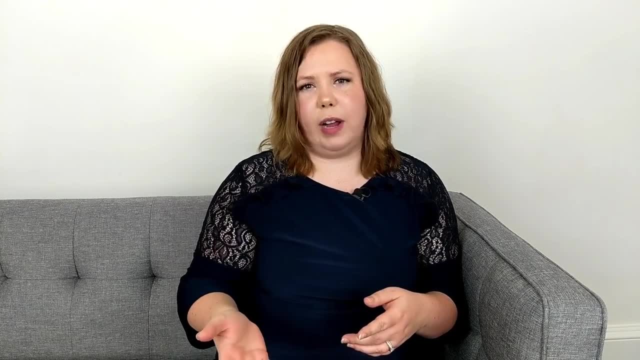 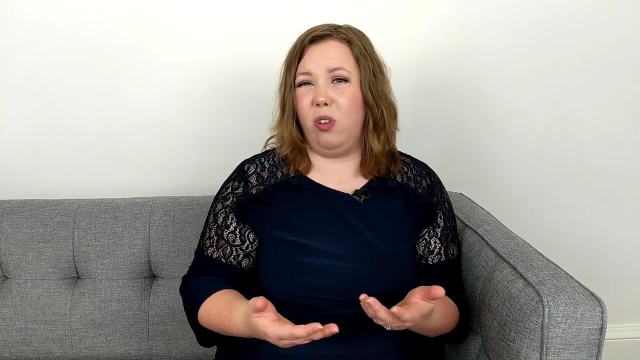 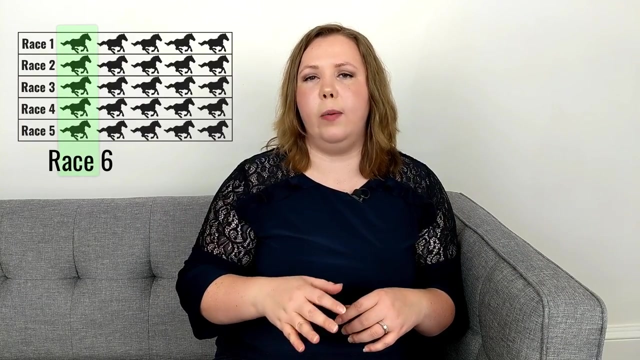 from each of those. but I would also need a sixth race because I only need to know the top three, and the top one from each doesn't tell me, because I don't know the times. I just know which one won, what order they finished in. So I would do a sixth race and that sixth race I would. 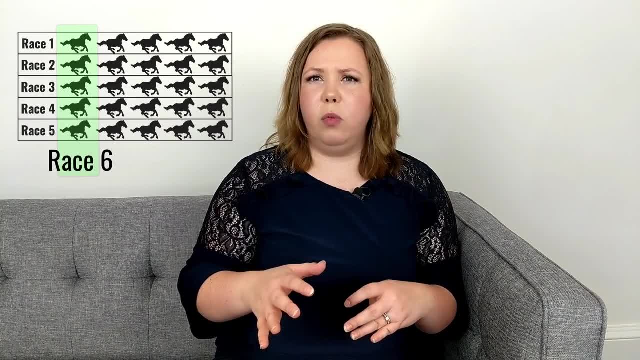 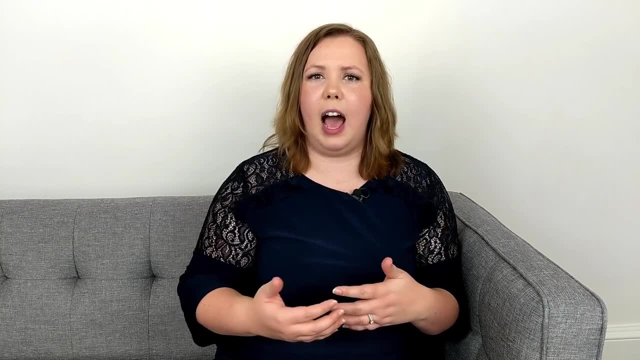 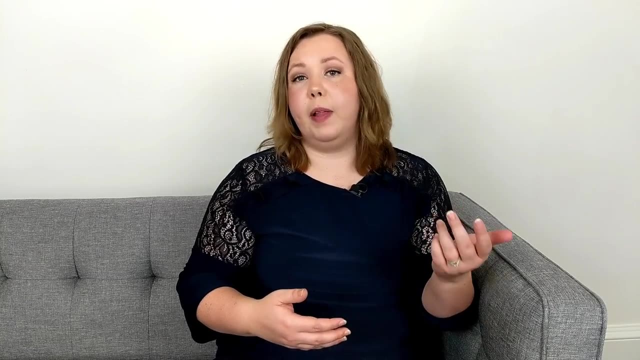 run the five fastest horses. That would tell me what the top three out of the top five were. but I would probably then run another race because I couldn't be sure that the fastest group that had the fastest horse didn't have a second place horse that was faster than the first. 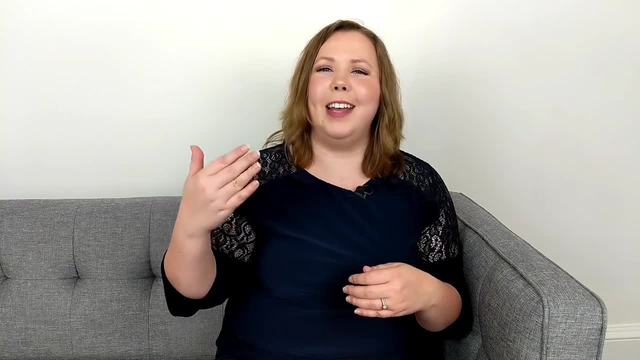 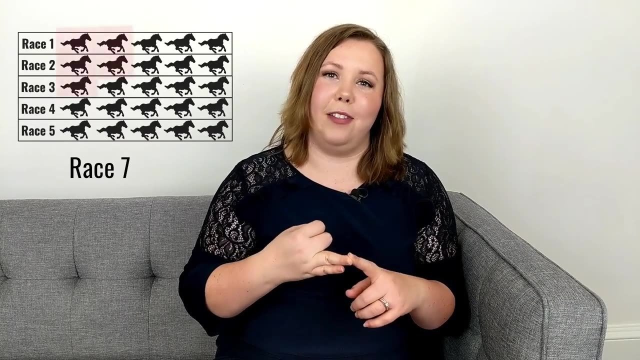 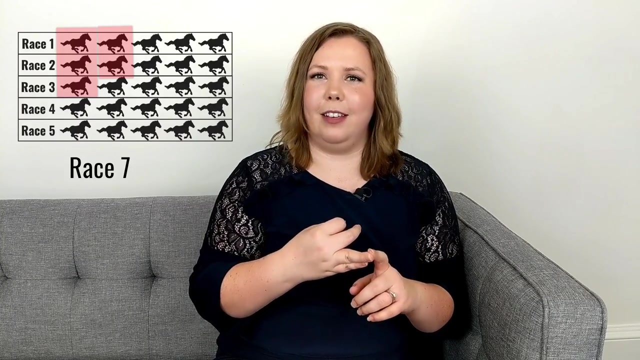 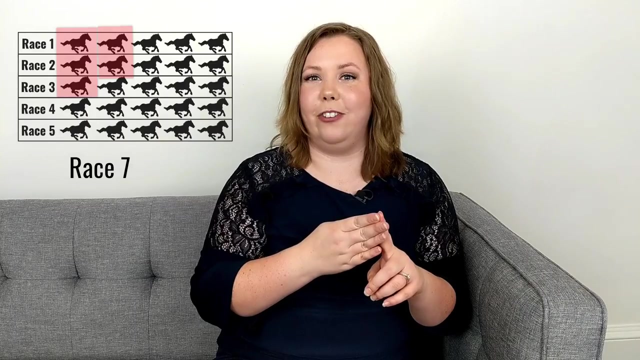 place horse in the second fastest group. So in that seventh race I would run the fastest horse, the second fastest horse from the same group as the first fastest horse, I would take the second place finisher from the sixth race. so the second fastest group, I would run that one and the second place finisher from. 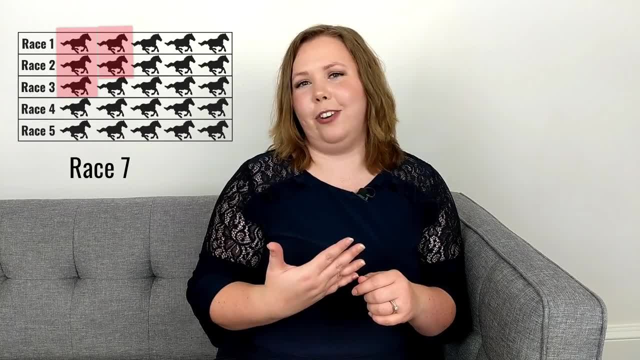 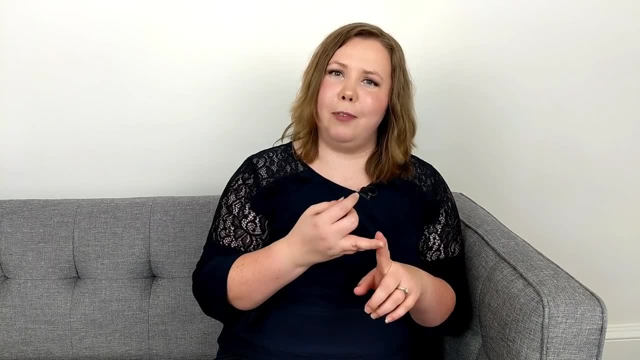 that group and I would take the third place finisher from race six and I would put that horse in the race. So that gives me five horses. That gives me the top two from the fastest group, the top two from the second fastest group. the fastest horse from the third group. So when I run those I would know whatever the three horses that finished first would be the top fastest horses out of the 25.. So I would say the minimum number that I need to run would be seven races to find the seven fastest horses, not knowing anything about their. 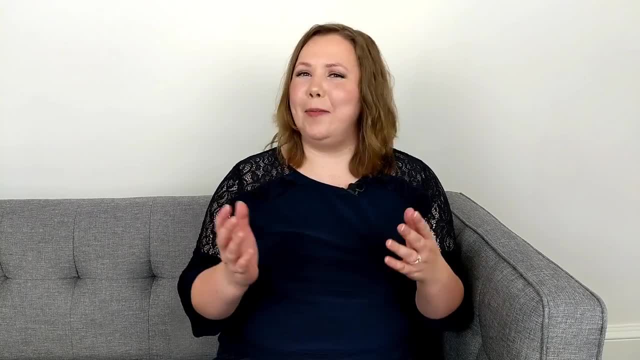 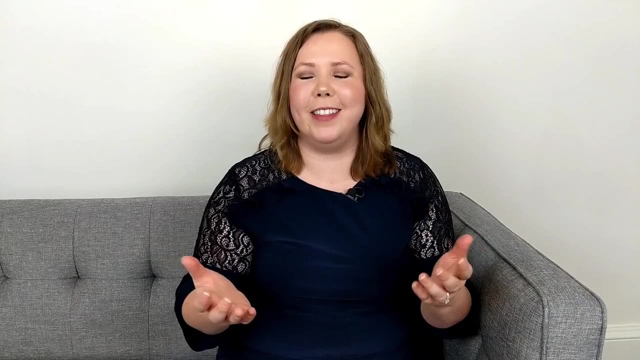 finishing time only knowing about their finishing place. I'm curious how well you followed along with that. Some of you probably thought, oh duh, this is obvious. and other ones of you probably thought I have no idea how I would have solved that problem. You know what? There are plenty of different problems, just like: 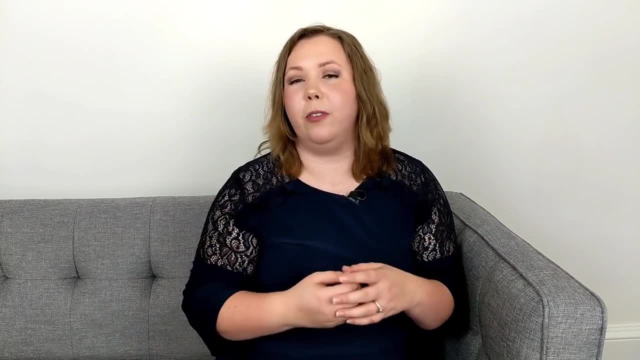 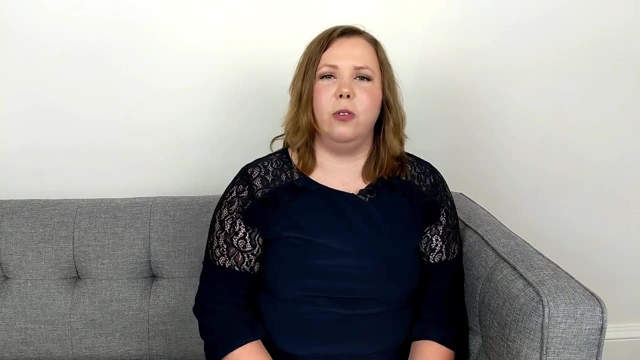 this. So if you want to practice, just google logical problems or analytical problems or puzzles- You'll find plenty of different ones out there that you can practice with. Whether it's other videos or just googling it, you'll be able to find some things to practice with. And the really important thing here wasn't 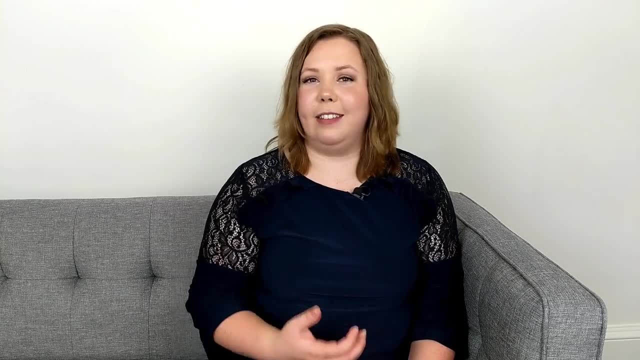 even the number of races that finished in first place, but it was the number of races that finished in second place. So you need to kind of necessarily that I came to the conclusion that I needed seven races to solve this problem. it was that I was able to explain my logic of how I got. 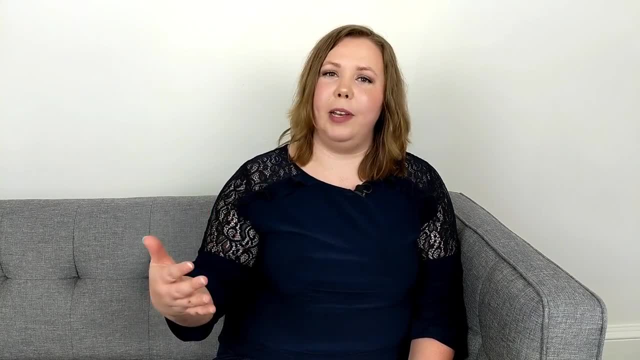 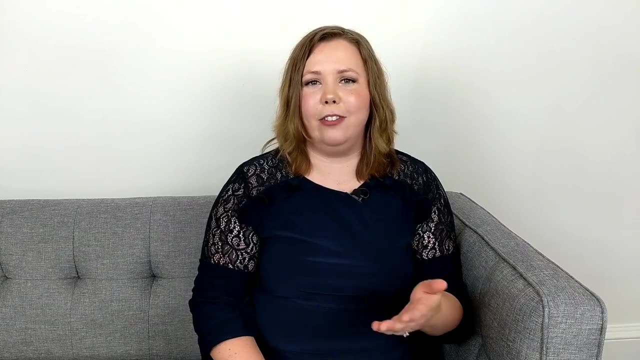 there. if I would have just responded to the question about how many races were needed and said oh, seven, and then just shut my mouth, then I haven't told the interviewer that much. they might be impressed that I knew it off the top of my head. or they might just think, oh well, she's heard this problem before, so she 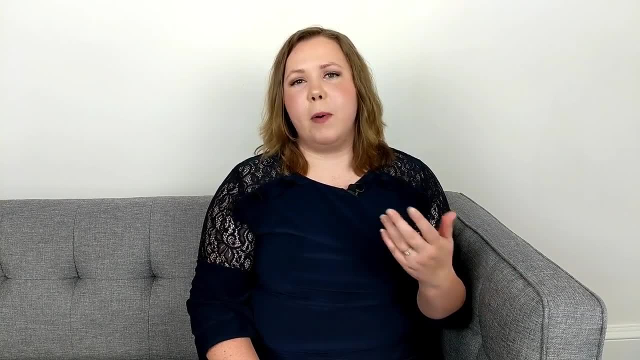 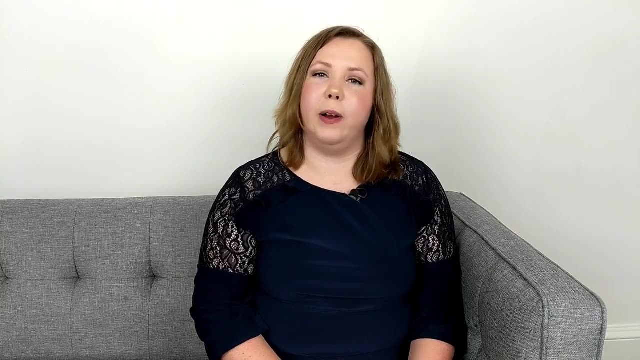 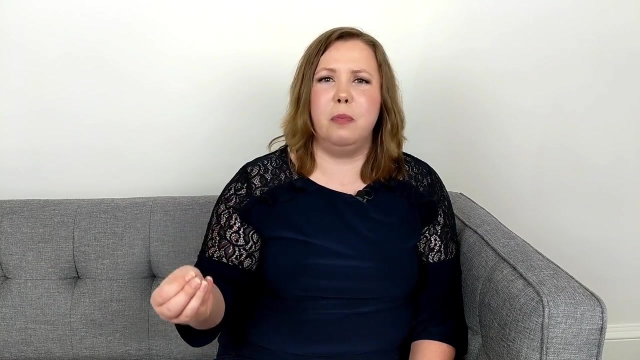 knows the answer. the interviewer really wants to understand what's the process that you go through to solve a problem, because as an analyst, that's so much of your job. that's really the value you're bringing is being able to solve these complex problems. the data and the math part of it are actually the smaller part. 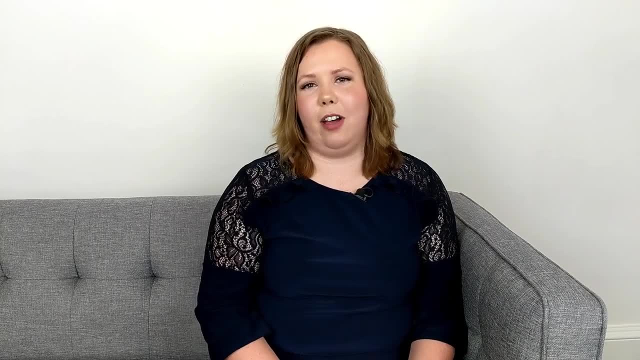 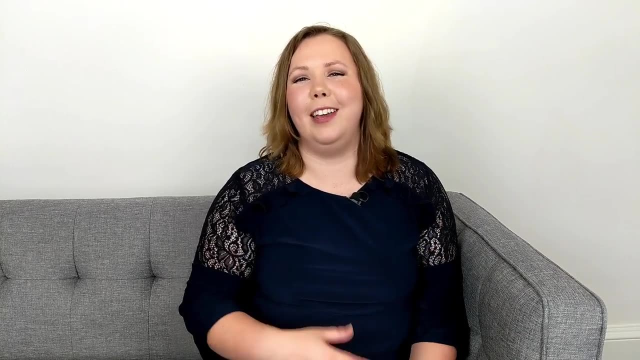 of the job that you're going to be doing, versus knowing how to actually solve a problem. there is one other place where you might encounter these problems, where you don't have a chance to really show your work, even if it's verbally. some employers now use logical screening problems. 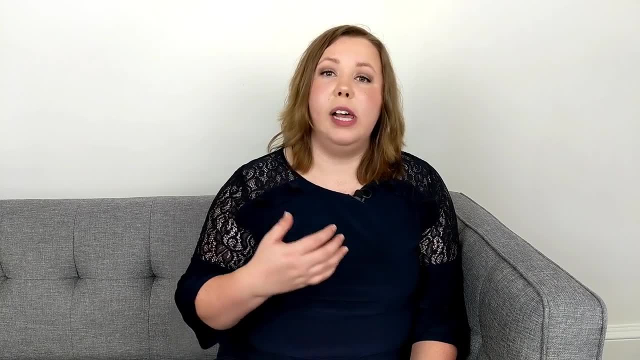 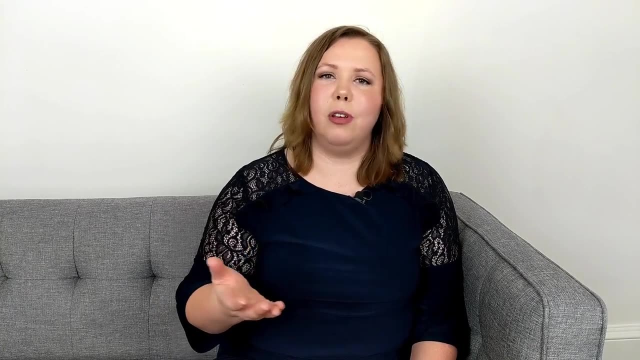 you might receive an email from a work in progress that says here's your schedule to pre-screen candidates before they have interviews. so typically how this works is you'll get a link to a website. you'll have a certain amount of time to go in and take a test- let's say typically 20. 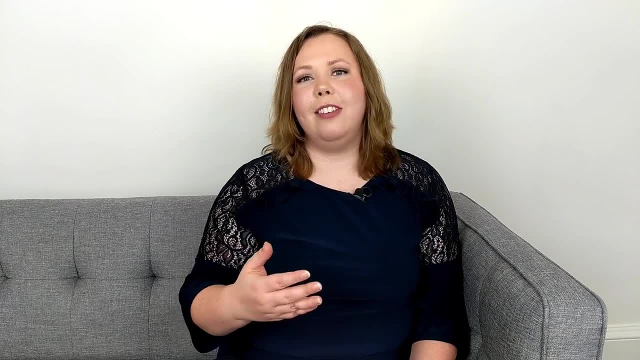 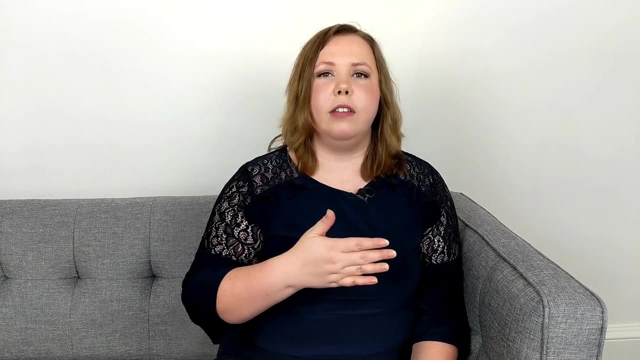 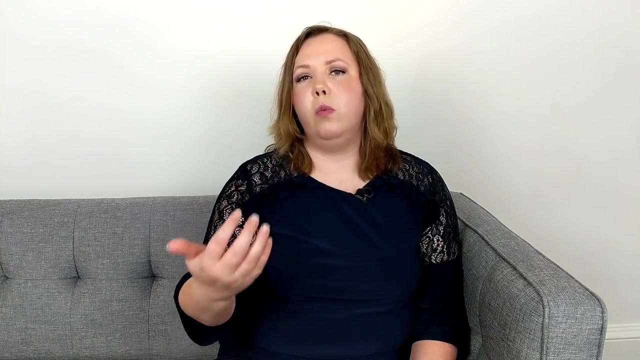 minutes to answer maybe 20 questions and in those cases you'll be given a series of things and asked to predict what comes next. so you might be given a series of squares that have different shading and you might be given four of them and ask: okay, now that you know these four, what?